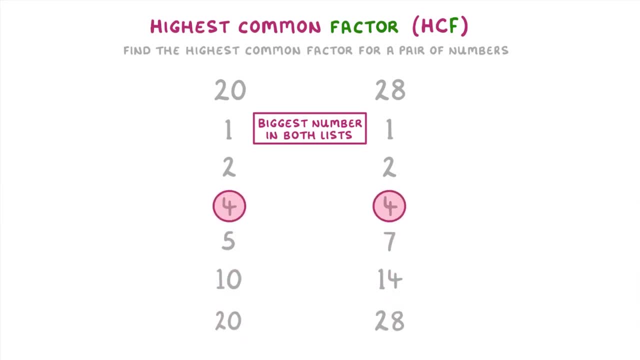 occurs in both of these lists, which is 4.. So 4 is the highest common factor of 20 and 28.. Have a go at doing the same thing for this one. So here we're being asked to find the highest common factor of 12 and 18.. So the first thing. 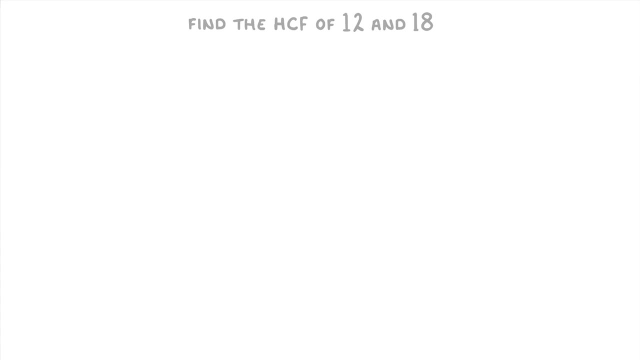 we do is list out all the factors of each, which are 1,, 2,, 3,, 4,, 6, and 12, and 1,, 2,, 3,, 6,, 9, and 18 for 18.. Then we just look for the biggest. 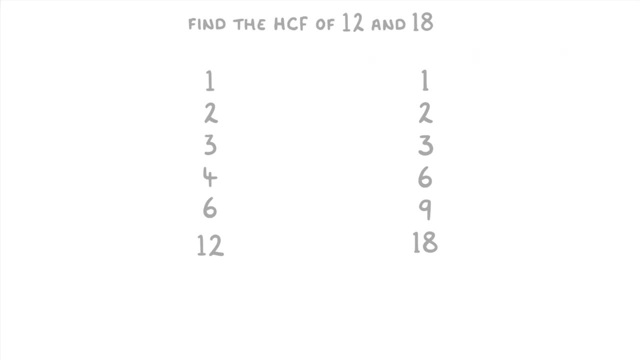 number that occurs in both lists. So that's going to mean 6 is the highest common factor, And that's all you have to do to find the highest common factor of a pair of numbers. We can also find the highest common factor using prime factors, The prime factors of: 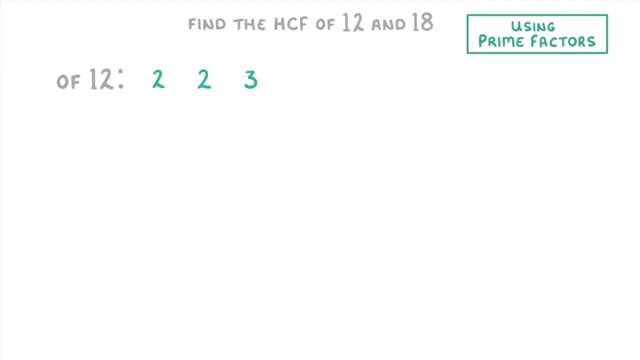 12 are 2,, 2, and 3,, because these are the prime numbers that multiply to make 12,, while the prime factors of 18 are 2,, 3, and 3.. Once you have the prime factors, to find the highest. 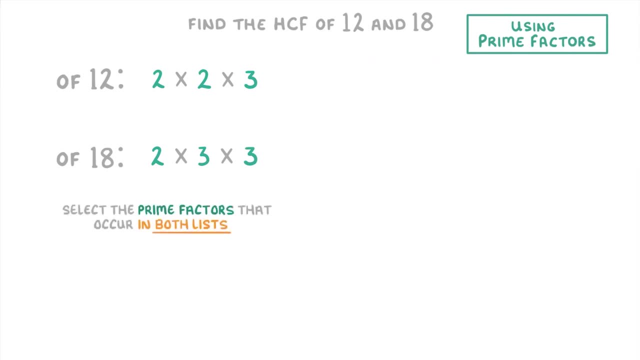 common factor. of the two numbers. you need to select only the prime factors that appear in both lists. So in this case that's a 2 and a 3. And we then multiply these together to get 6,, which will be our highest common factor. 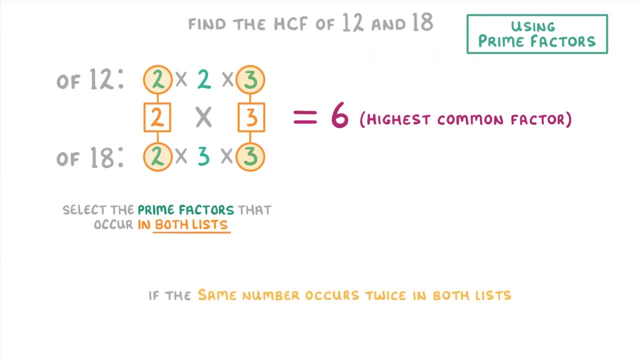 Now if the same number occurs twice in both lists, then we're going to have to include it twice. For example, let's change the 18 to a 20,, which has the prime factors 2,, 2, and 5.. 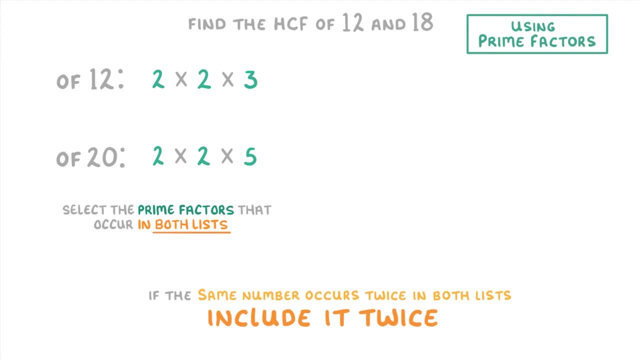 This time, the prime factors that appear in both lists are these 2s and these 2s, So we're going to have to multiply 2 times 2 together to get 4 as our highest common factor. Try using this technique for this one.